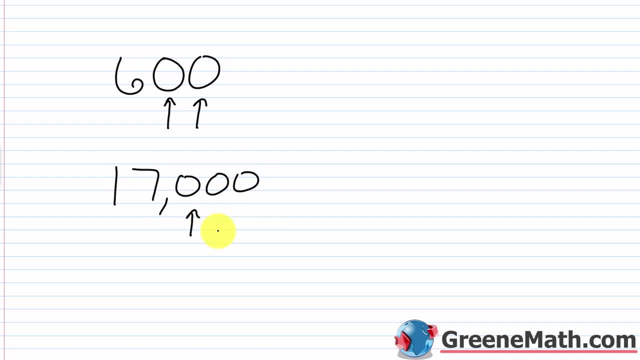 at the number 17,000.. This number has three zeros at the end of it, So it has three trailing zeros. Where people get confused is you might have a number like I don't know, let's say 104,030.. 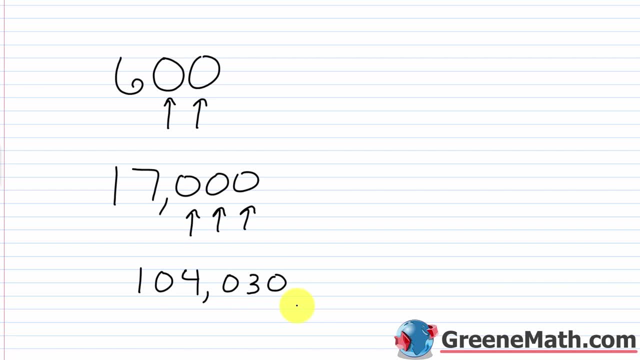 This number has three zeros in it, but they're not all trailing zeros. You're only looking at three trailing zeros, So you might have a number like I don't know. let's say 104,030.. Zeros at the end of the number. It can't be interrupted by something that's not zero. So 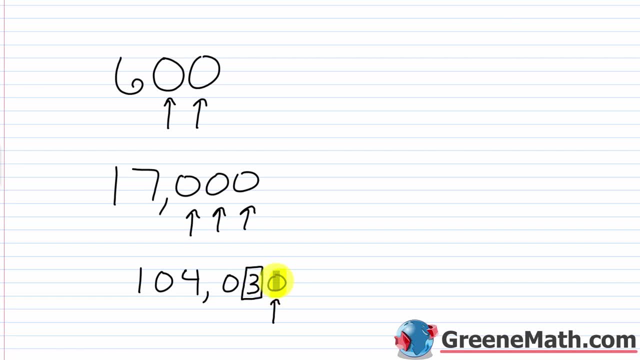 this one right here at the very end. that's a trailing zero, But because there's a three here, you can't say that this is a trailing zero also. Yeah, it's close to the end of the number, but it's not at the end. It's interrupted by this three here, So this number would have. 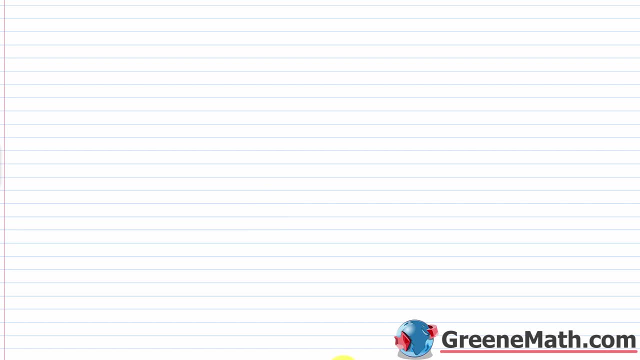 one trailing zero. Let's think a little bit about a simple multiplication fact that you might not have ever thought of. When you multiply, let's say something like five times 10.. We know that this is 50. But another way to attain this. 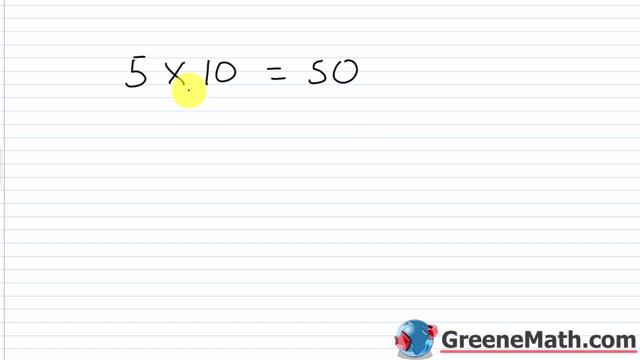 result is to multiply the non-zero parts. So five times one. that would give you five, And then just attach the trailing zero to the end of the result. So in other words, I can do five times one And then I can attach a zero to the end. that would give me 50. And I would have the result. 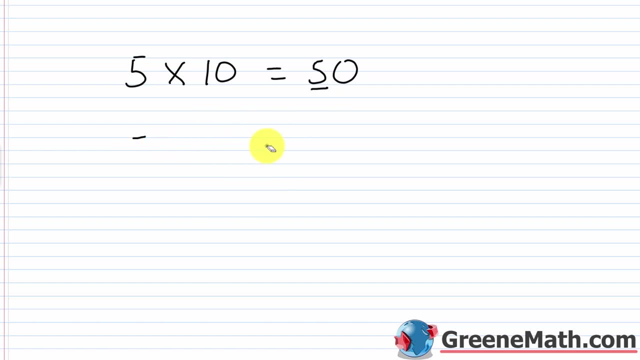 for five times 10.. And this works no matter how large your numbers are. Let's say I would have said: what is five times 100?? Well, now I would do five times one, that's five. And then I would attach two zeros to the end, two zeros to the end to get 500.. Let's say I did five times 10,000. 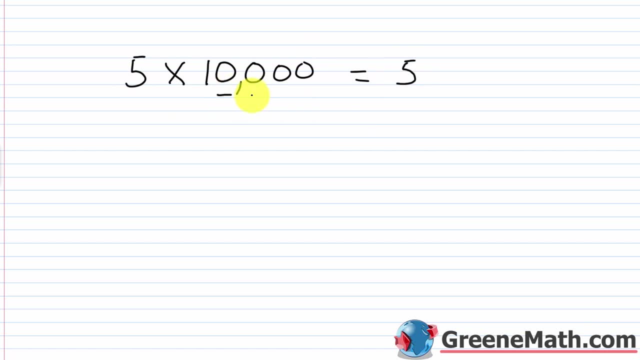 I'd do five times one, that's five, And I'd attach one, two, three, four zeros to the end. One, two, three, four zeros And I'd get 50,000.. Okay, So it's a simple multiplication fact, But once we learn it, 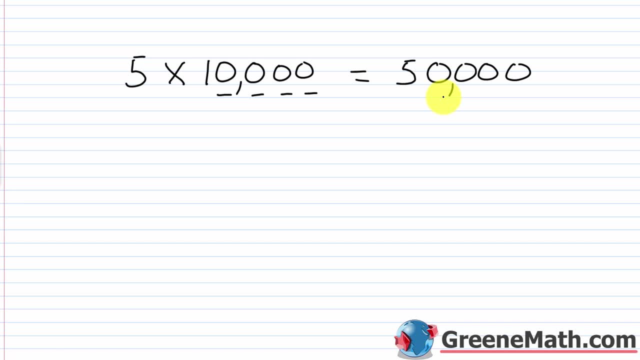 and understand how to use it, it can greatly speed up our multiplication. You'll come across a lot of problems with trailing zeros and you might not have a calculator to use, So this is a trick that can speed you up significantly. So just to look at the official procedure, essentially you just 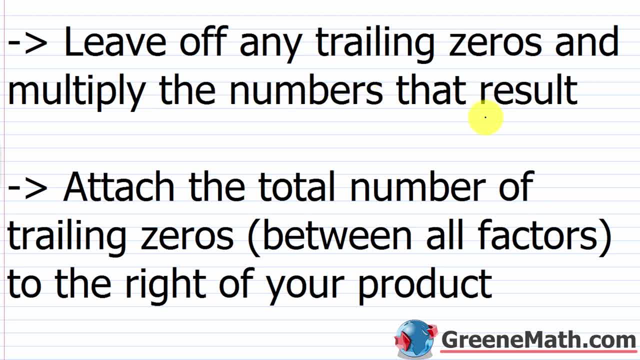 want to leave off any trailing zeros and multiply the numbers that result, And then next you want to attach the total number of trailing zeros And this is between all of them, And then you want to add all factors to the right of your product. So again, super, super easy to do. Let's just look. 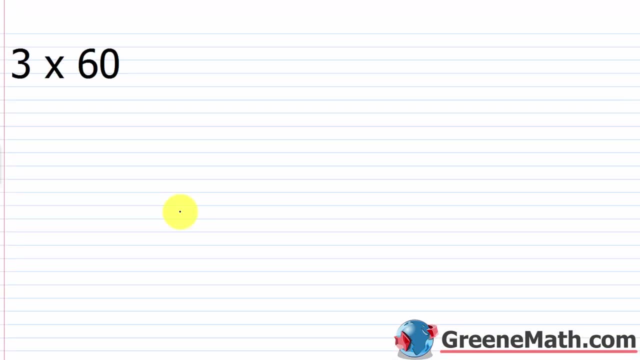 at some examples. All right, So let's start out with three times 60. So we want to multiply and leave off the trailing zero. in this case, What would three times six be? That's 18.. And then all we need to do is attach the total number of trailing zeros between all factors. 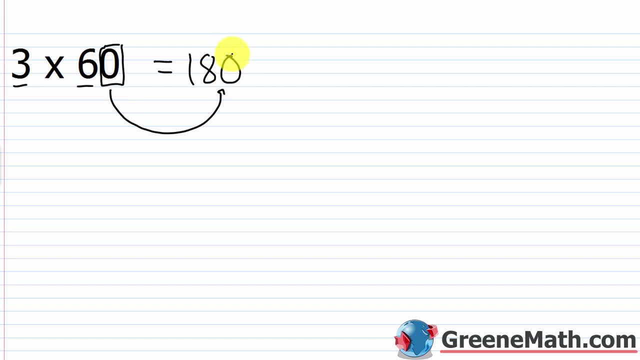 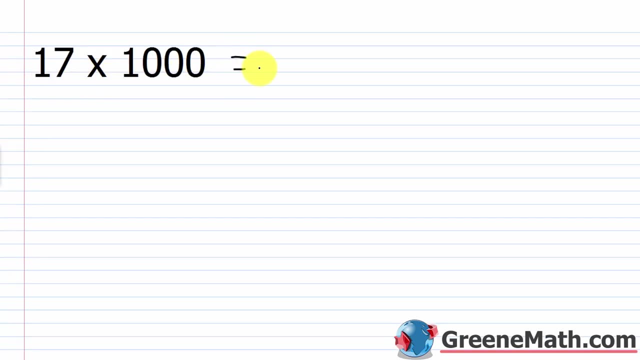 in this case, just one to the end of that number. So we end up with 180, and of course that's correct. 3 times 60 is 180. what about 17 times 1000? well, we'd multiply 17 times 1. right, you would leave this part off. these are the 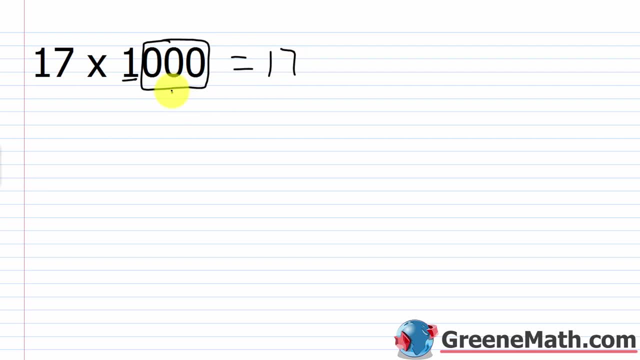 trailing zeros. 17 times 1 is 17, and then you would just attach them to the end of the number. I have 1, 2, 3 trailing zeros, so I write 1, 2, 3 zeros there, and so 17 times 1000 is 17,000. all right, let's look at an example where both numbers 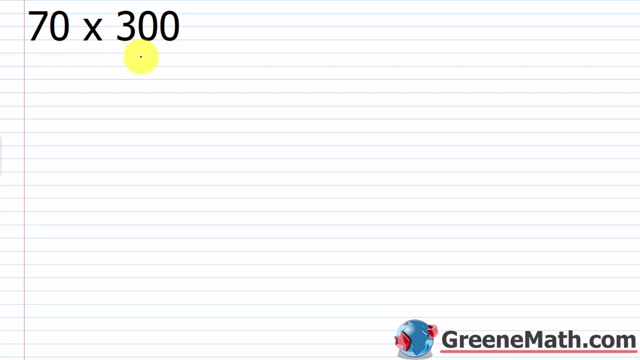 have trailing zeros. here we have 70 times 300. so 70 has one trailing zero, 300 has two trailing zeros and essentially just leave those off. leave those off and you would do 7 times 3. 7 times 3 is 21, and then I'm going to. 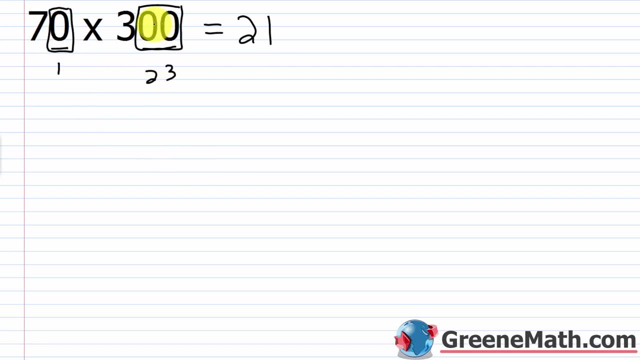 attach 1, 2, 3 zeros to the end, because that's how many trailing zeros there are between all the factors. so 1, 2, 3 trailing zeros are attached, and so 70 times 300 is 21,000. okay, what about 153 times 9,000? so a lot of us cannot do. 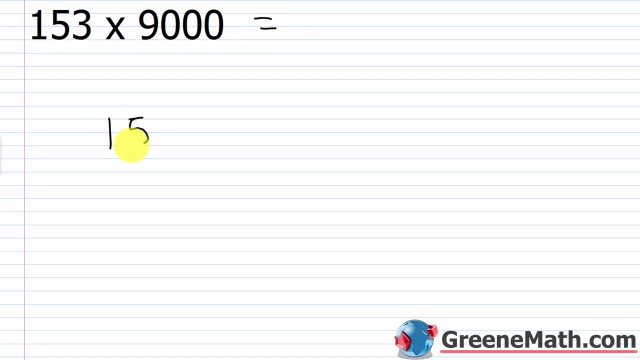 153 times 9 in our head. I'm going to do 153 times 9 in vertical multiplication format and then, when I'm done, I'm going to take this result, bring it up here and attach three zeros to it. all right, so 9 times 3 is 27. put a 7 down, carry the 2. 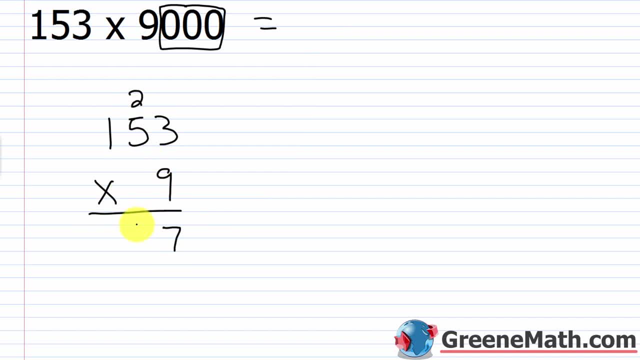 9 times 5 is 45 plus 2 is 47. put a 7 down, carry the 4 9 times 1 is 9 plus 4 is 13, so I get 1377, so 1377, and I'm just going to attach three zeros to the end of that: 1, 2, 3, comma, comma and so. 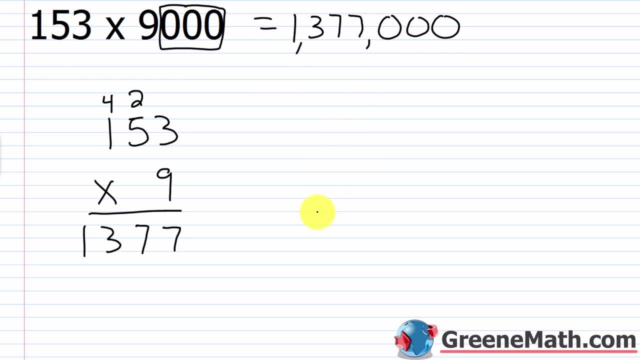 our result is 1,377,000. okay, let's look at another one. we have 216,000 times 108,000. so we have three trailing zeros here and we have three trailing zeros here. so I'm just going to multiply 216 times. 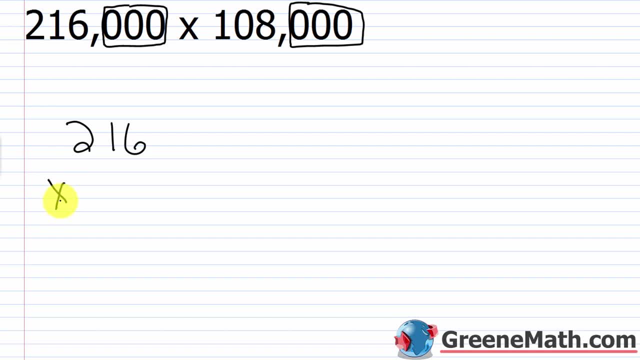 108, 216 times 108, and when I'm done I'm going to attach one, two, three, four, five, six, six zeros to the end of whatever the result is from that. so eight times six is 48, put an 8 down, carry a 4. 8 times 1 is 8 plus 4 is 12. put a 2 down, carry a one. 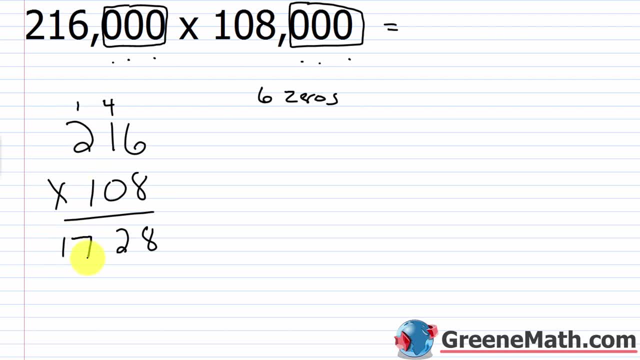 eight times 2 is 16 plus one is 17.. Zero times 216 is zero. So I can put a zero here or I can leave it off. doesn't really matter, I'm just gonna leave it off. And next we move to this one here. 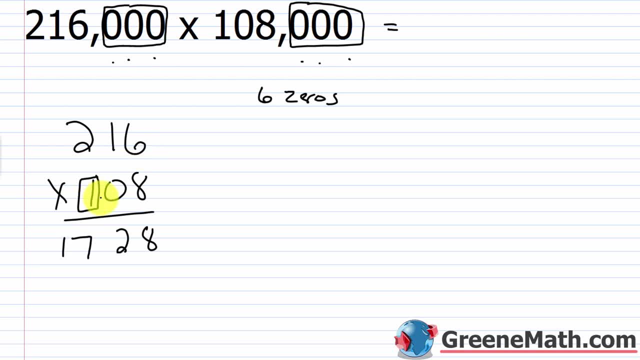 I have one times 216.. Remember, the one is in the hundreds place, so I have to start my answer in the hundreds place. And one times anything is just itself. So one times six is six, one times one is one and then one times two is two. 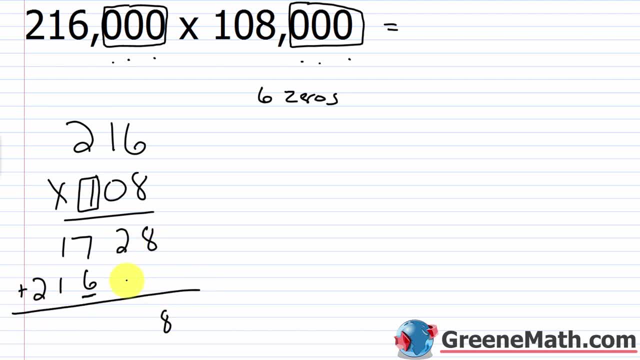 So we find our sum. bring down the eight, bring down the two. seven plus six is 13.. Put a three down and carry the one. One plus one is two, two plus one is three. Then bring down this two and we get 23,328.. 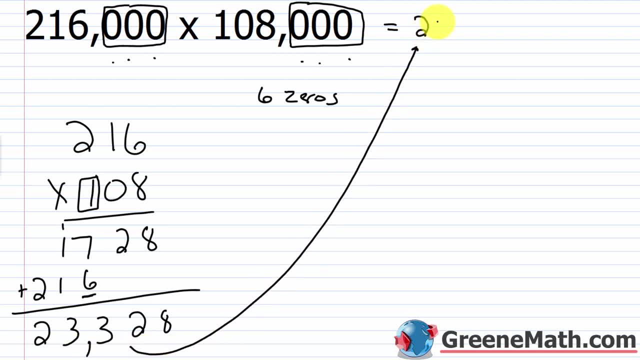 Now I'm gonna bring this guy up here- 23,328. And I'm going to attach six zeros to it. So let me actually write it a little bit lower: 23,328, one, two, three, four, five, six. 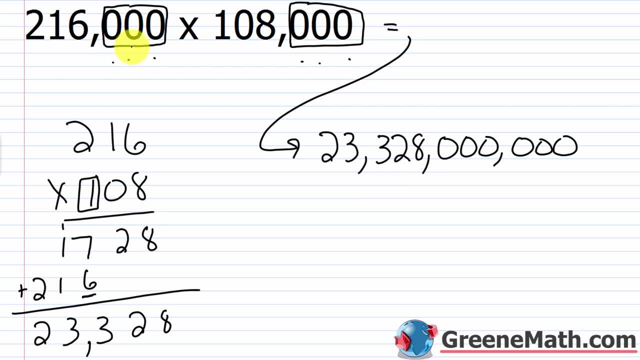 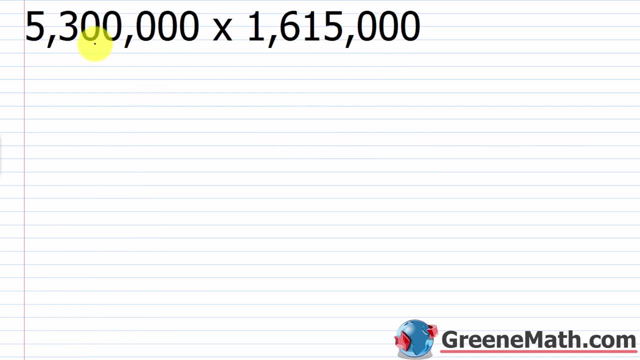 So this is our answer for 216,000 times 108,000.. We get the result of 23,328,000,000.. For the final problem, we have 5,300,000 times 1,615,000..